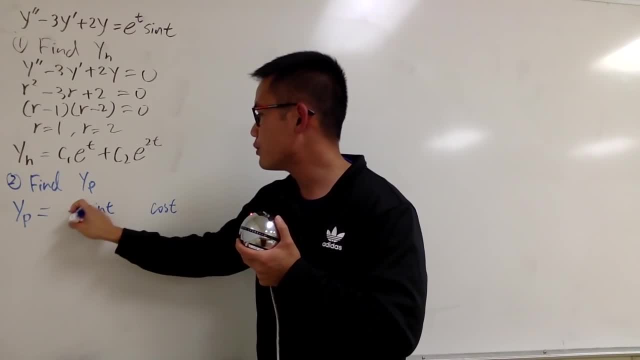 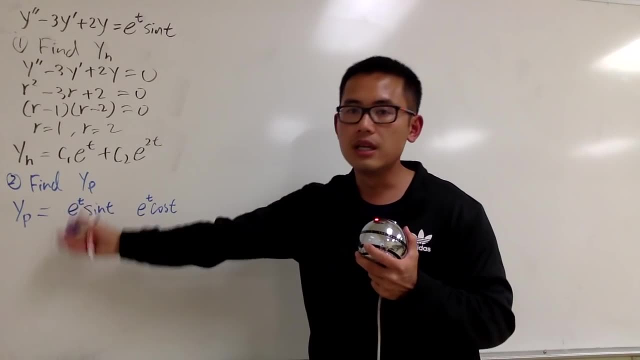 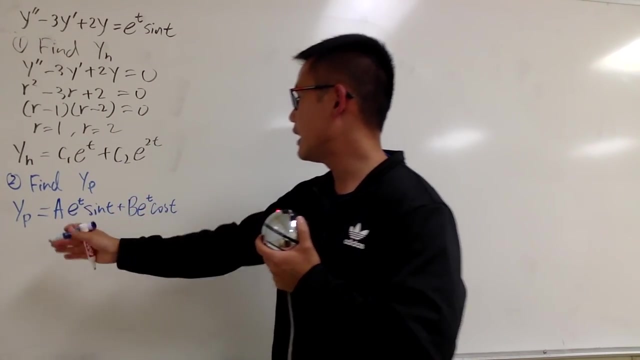 And this is being multiplied with e to the t. so, right here, I will have to multiply this by e to the t. likewise here, e to the t. okay, So this is pretty much a building block for this particular solution. But I don't know the co-efficient though, so I'm going to put down a right here, b right here, and then I'm going to add them up. 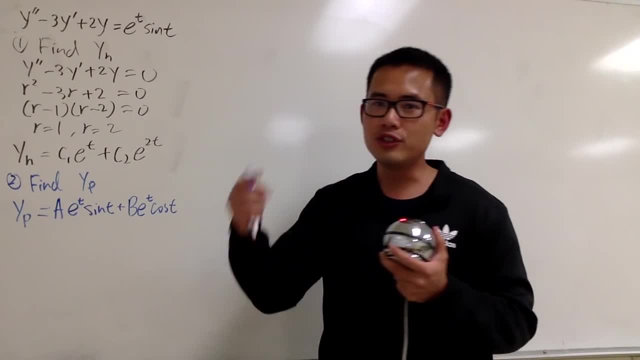 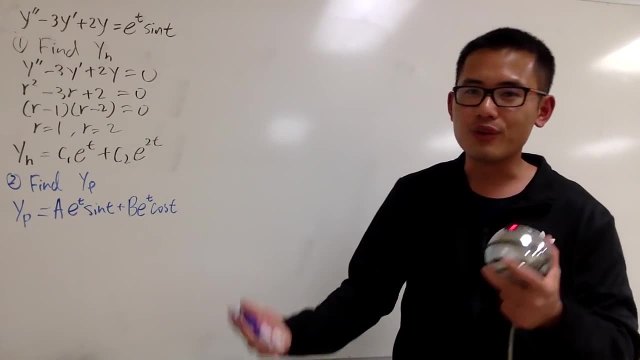 So you know the deal. We take this and differentiate twice and then plug in the second derivative and the first derivative and also the original into the differential equation and then match the coefficients and then find out what a and b are right. 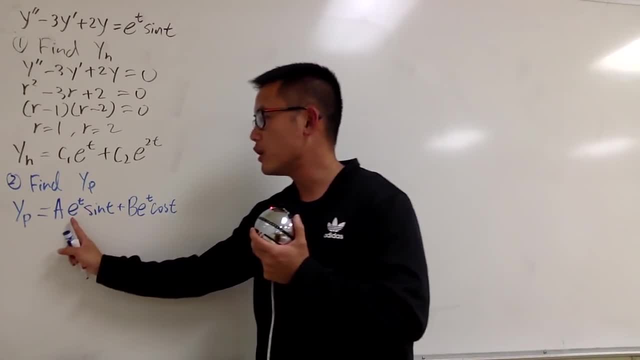 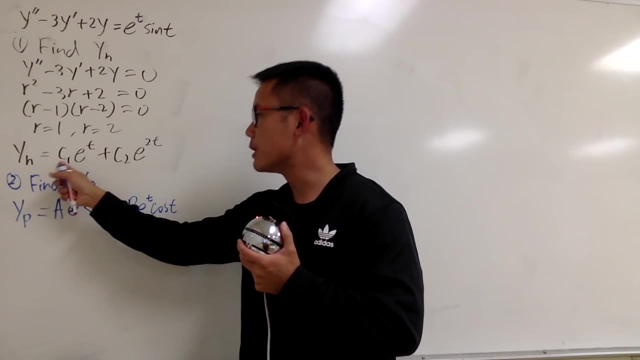 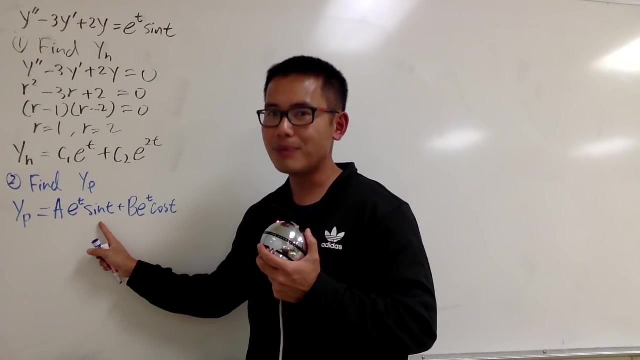 And another remark before we do that. you see, yes, here we have e to the t and yes, here we have e to the t as well, but this is just a constant multiple with e to the t. Right here we have a times e to the t, and this is also being multiplied by sine t. 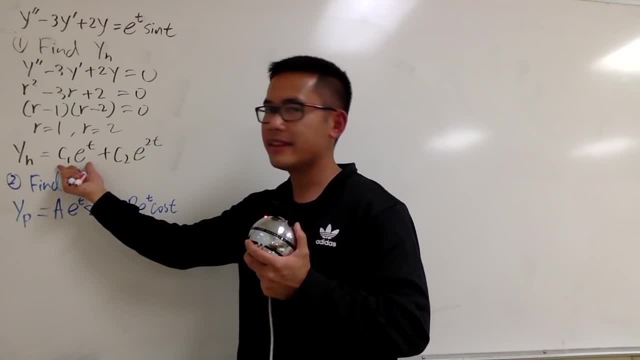 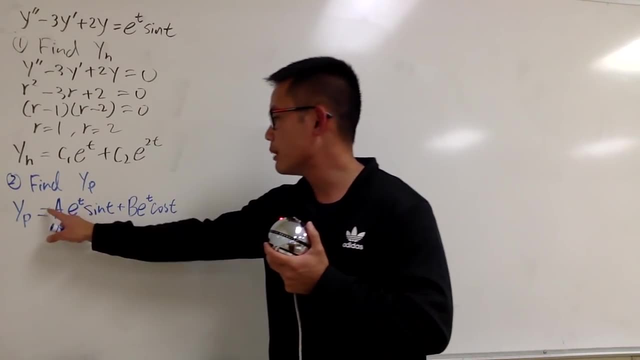 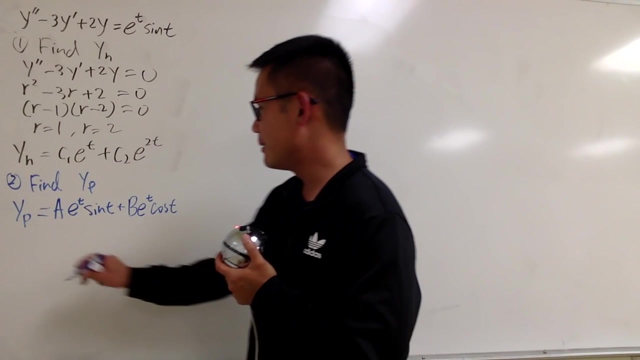 In another word this, and that they are not a constant multiple of each other. This and that are linearly independent, so we don't have to multiply by any extra t right here, which is a great news, isn't it? Anyways? derivative in action: yp', and let me just put this down like this: 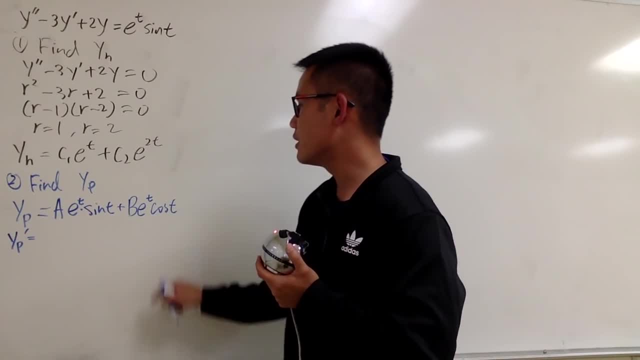 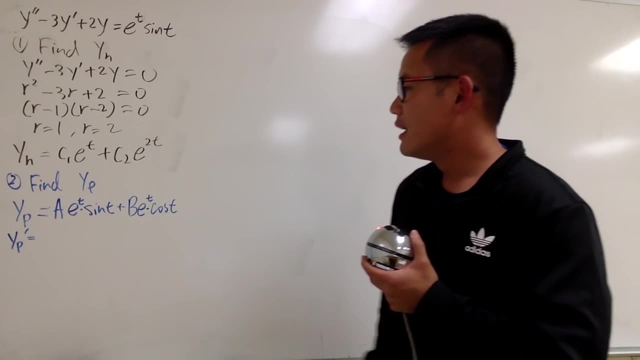 I will look at this as my first function, and then this is my second function, and likewise for the second term. this is my first And that's my second. You know we have to do the product rule right. Anyways, right here, I'm going to first keep my first function, which is a e, to the t. 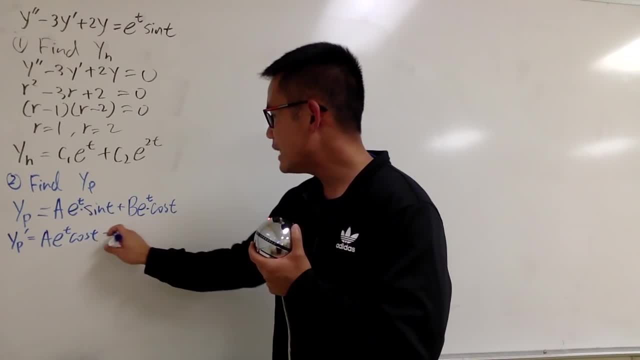 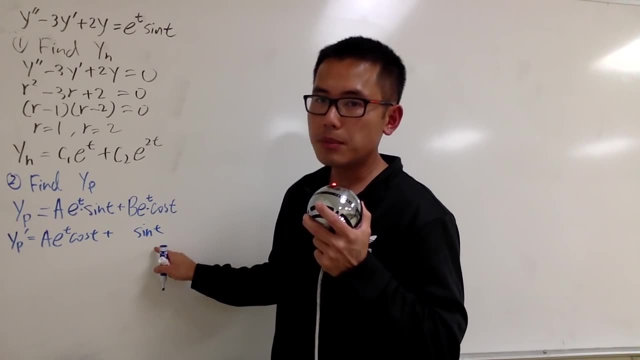 and the derivative of sine is cosine t, and then we add it with the, we keep the second function, which is sine t. so let me put it down right here, okay, And we multiply by the derivative of a e to the t, which is just a e to the t, okay. 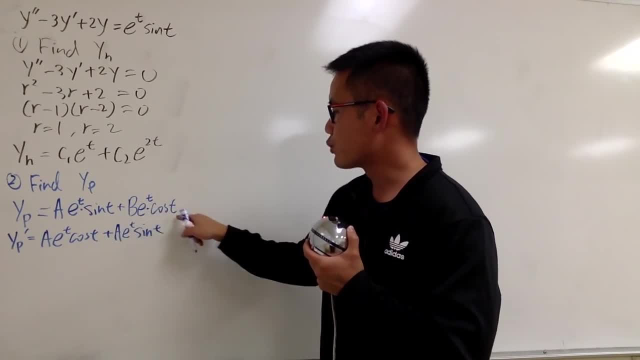 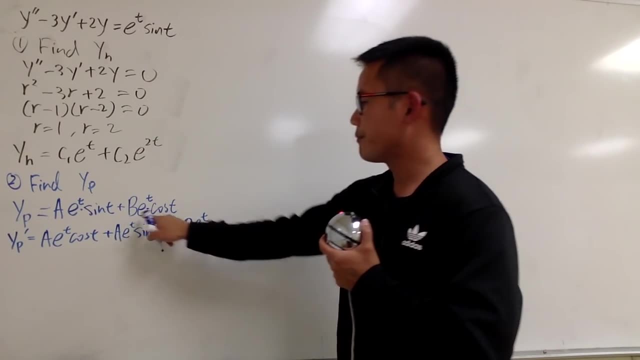 And the next. we are going to be using a product rule right here as well, so I will put down. well, let me just put down the first function right here, which is b, e to the t, and I will multiply by the derivative of the second. 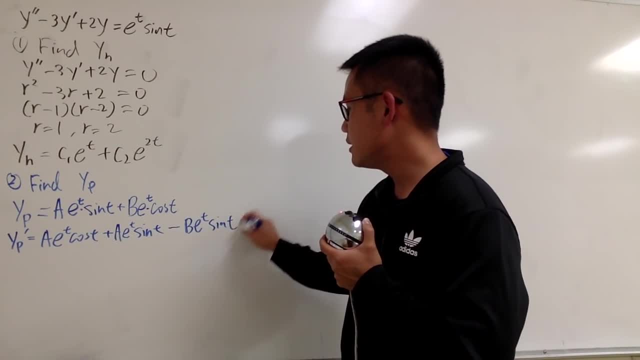 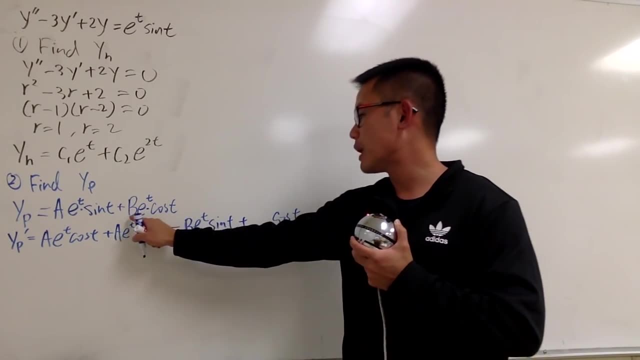 The derivative of cosine t is negative sine t. okay, So we have the subtraction right here And we add the second function, which is cosine t, and multiply by the derivative of the first. The derivative of b? e to the t is just exactly b? e to the t, and that's such a beauty. 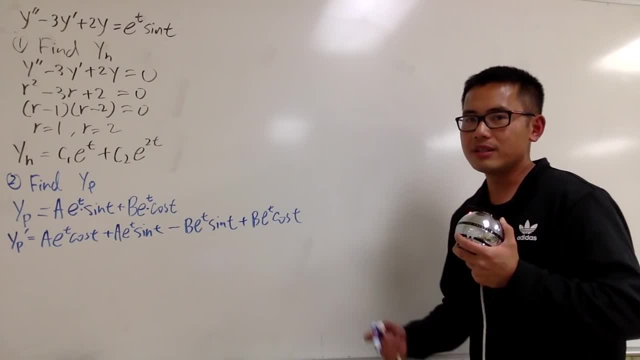 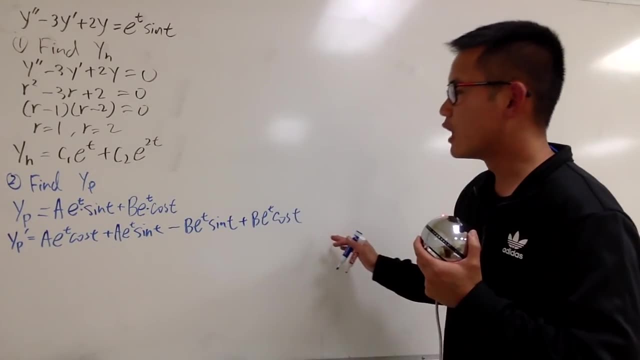 Anyways, this is what we have And if you would like, you can kind of combine the constants for the a and b. Maybe you should do that, because right here we have four terms already And you know this is multiplying, right. 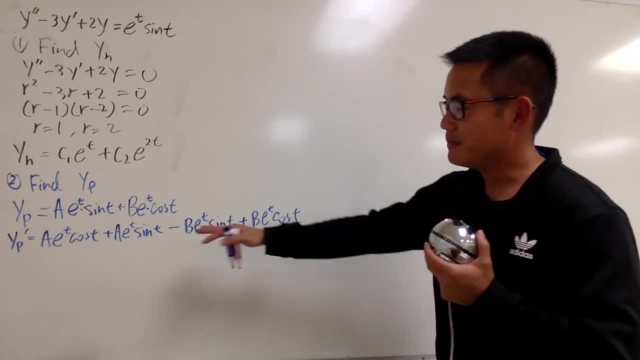 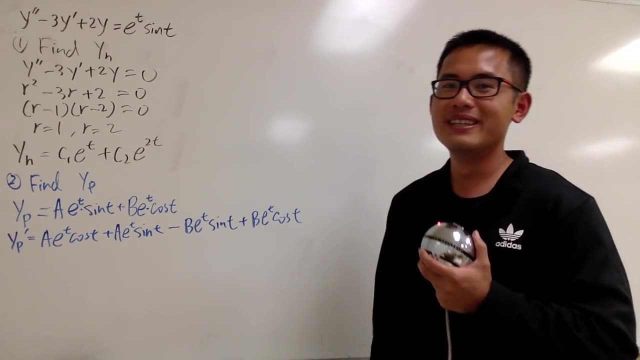 They are multiplying, so two functions. If you want to just look at the expression like this as how it is, and then do the derivative, you know you have to use the product rule four times and you end up with a really long expression for the second derivative. 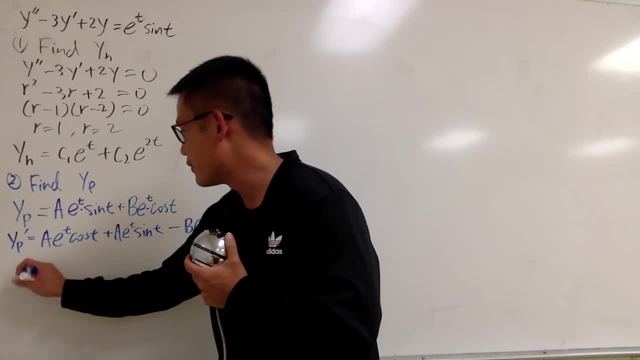 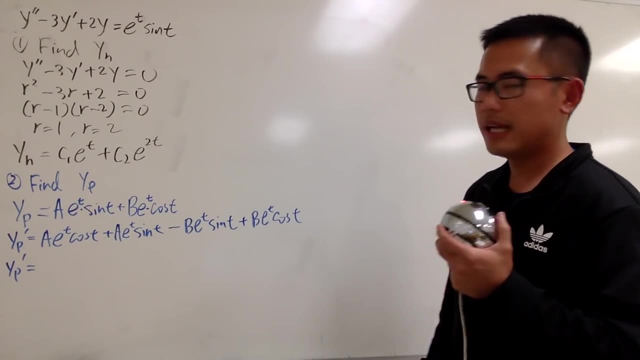 So, seriously, we should just like collect some terms before we do the next derivative. This is still my first derivative, okay, So what I would like to do is let me collect all the terms that has e to the t times sine t. 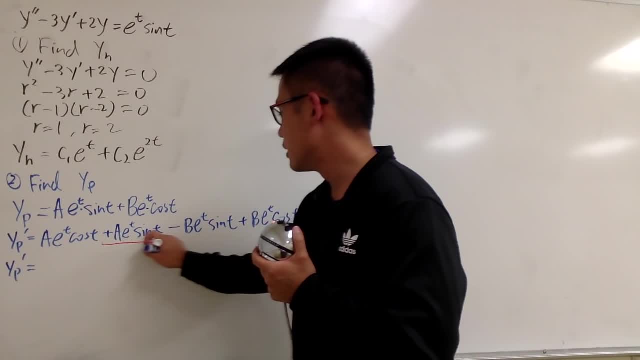 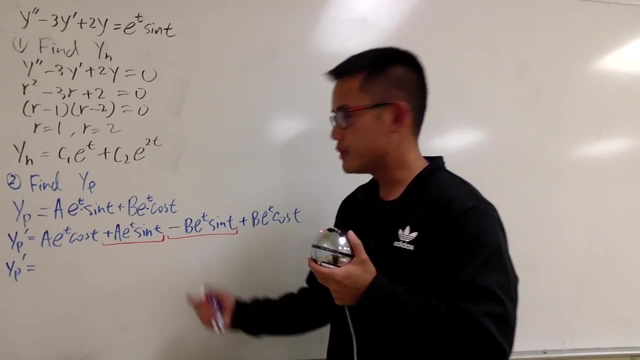 So I'm talking about this one right. This is a term that has e to the t sine t, And likewise we can also combine it with this. Well, I'm just going to put down the function part right here: e to the t times sine t. 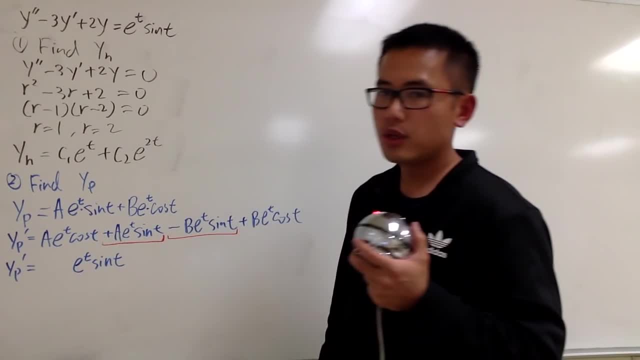 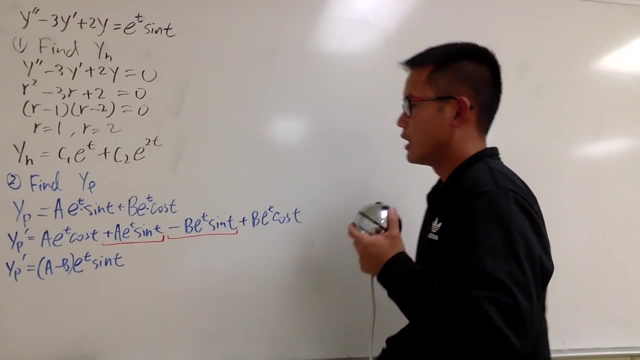 Well, I'm just going to put down the function part right here: e to the t sine t and the coefficient is a minus b, right? So let me just put it down like this: a minus b, like that Cool. 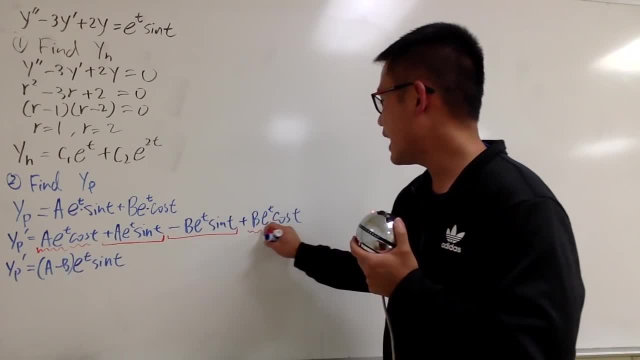 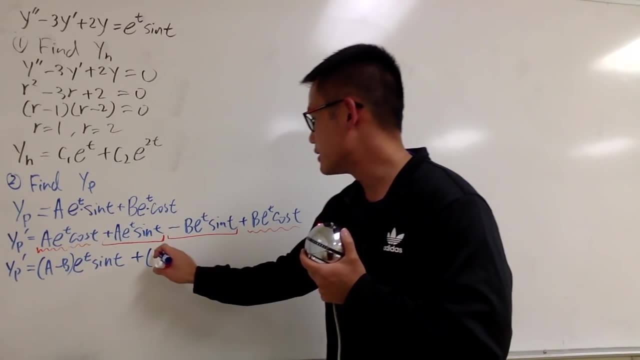 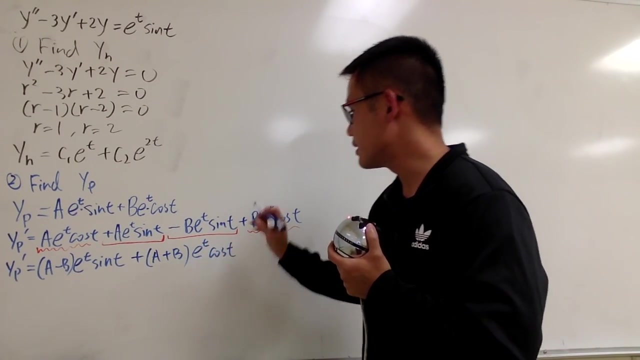 And then you see this and that can be combined as well. I will be adding them together. The coefficient is a and the coefficient here is b, so it's a plus b, And then I will put down e to the t right here: times cosine t, like this: 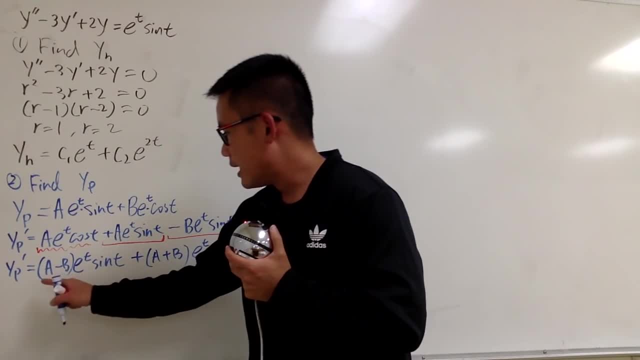 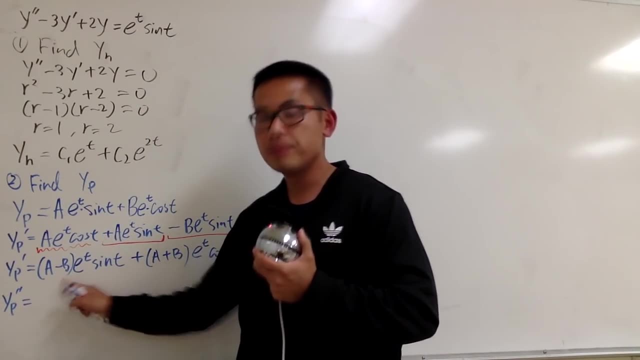 Okay, Okay, Okay, To do the next derivative. once again we are going to use the product rule. And now you know a minus b is just a number. Do not put that down. say another constant. We must have a and b together like this: 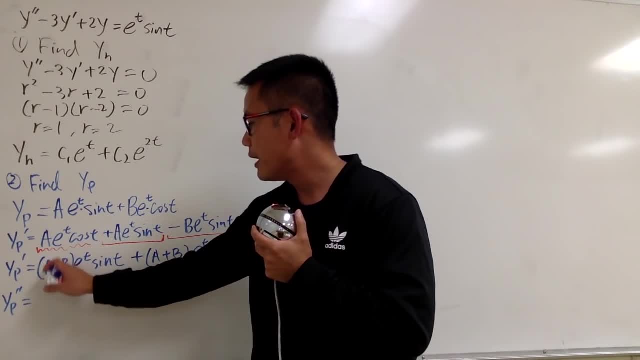 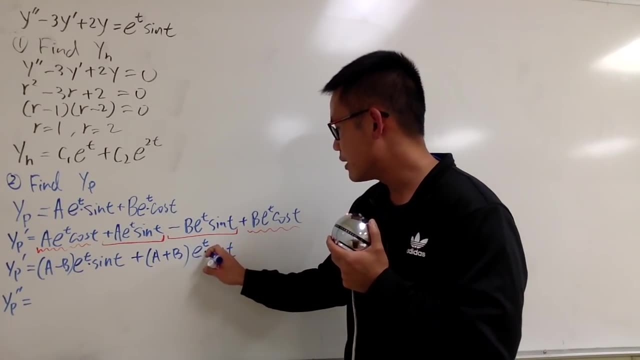 Okay, We have to work with a and b. I'm going to just pair up a minus b times e to the t as the first function and sine t will be my second. Likewise, I will do the same right here, And this is just a. you know, dot for multiplication. 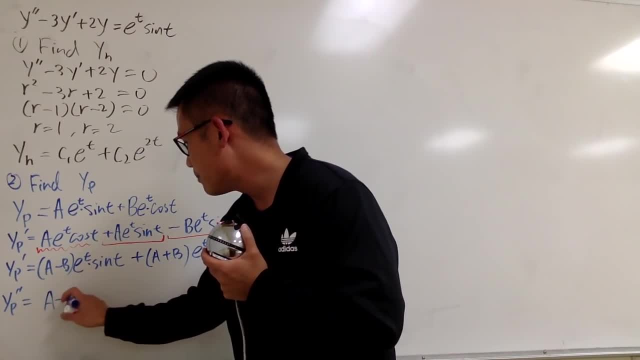 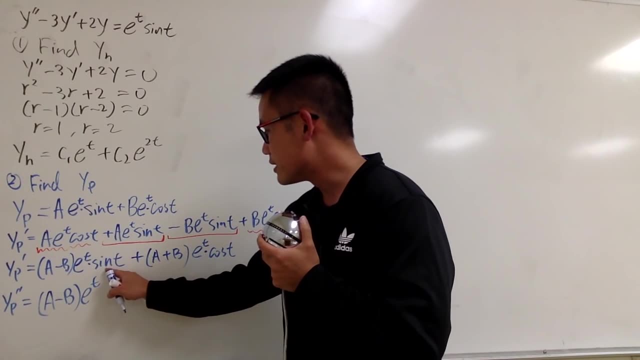 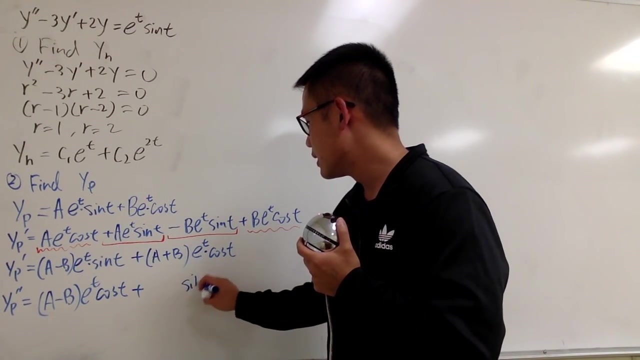 Here we go. Here we go going to keep the first function, Namely, I will put down a minus b times e to the t. This is technically my first function, And then I will differentiate the second function, which is going to be cosine t, And I will keep the second function, which is sine t. 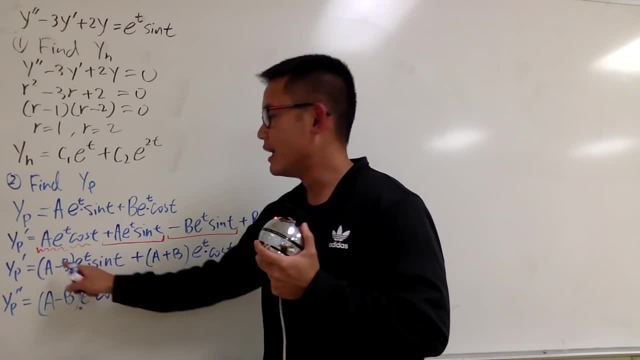 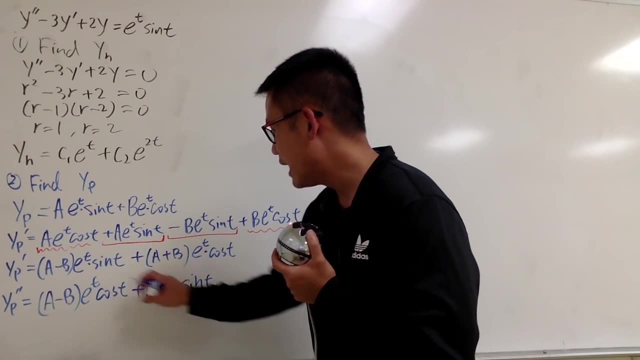 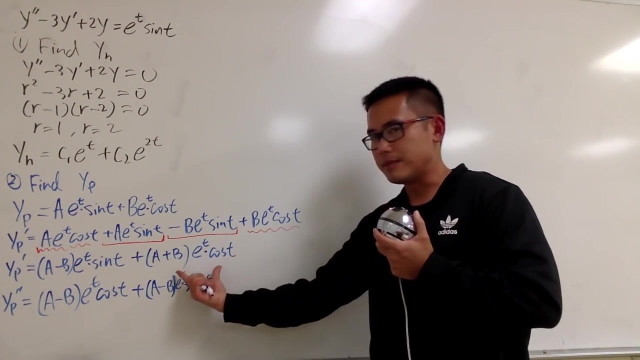 And then I will differentiate the first. The good thing right here is that the derivative of the first is just that, because it's a constant multiple of e to the t, So it will still be a minus b e to the t, like this. okay, And then we'll do the same thing, right. 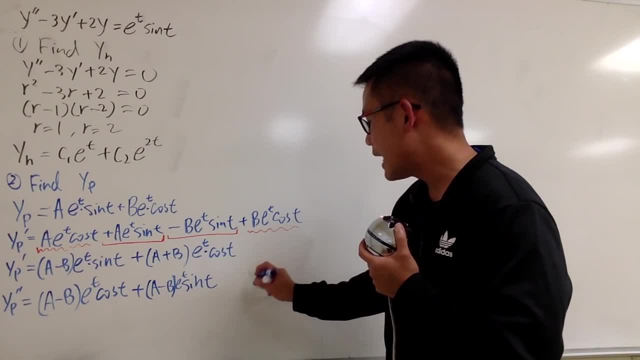 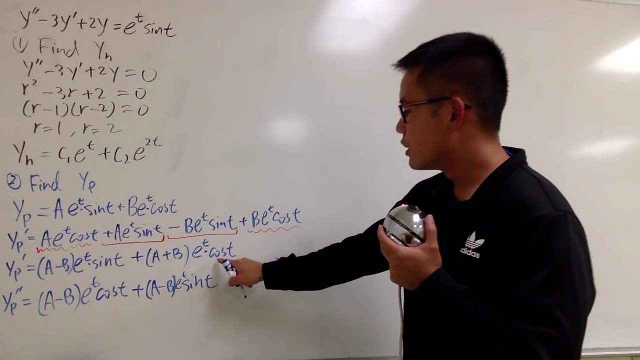 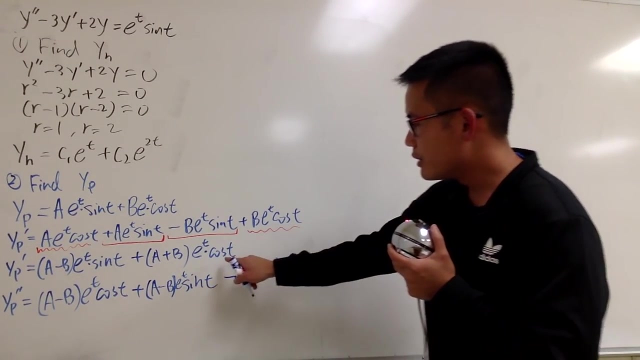 here. I'm going to first keep the first function, so I will write down a plus b, e to the t, okay, And we'll differentiate cosine, which is going to give me negative, sine t, like that. And I will keep the second function, so I'll put it down right here: cosine t. 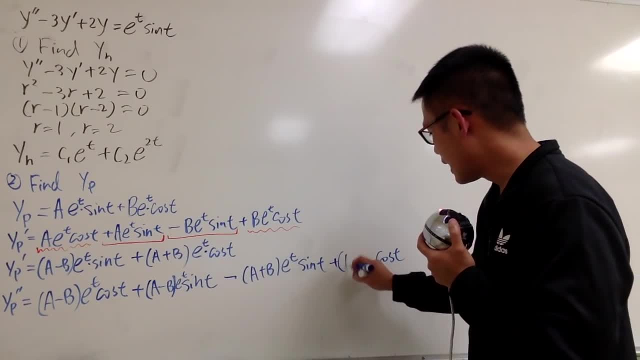 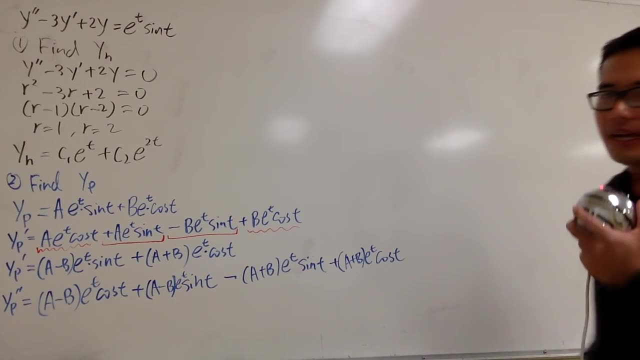 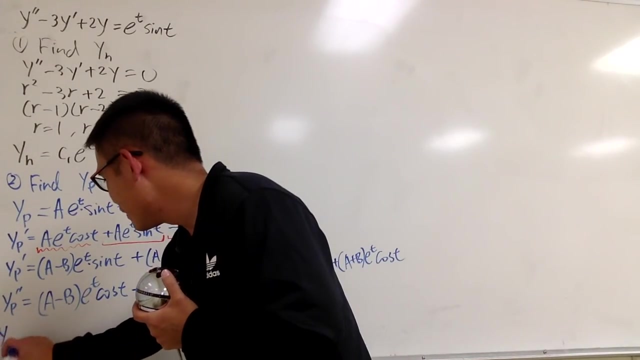 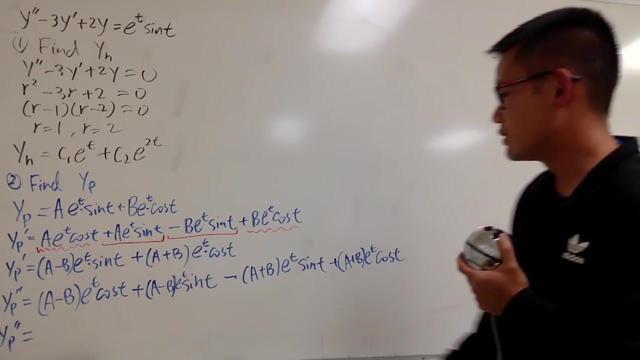 and we'll differentiate this, which is still that right. So we'll have a plus b e to the t, just like that. That's the second derivative. And can we combine terms? Yes, we can, right, y, p, double prime. This is going to be. let's work with the e t sine t first, which is once again. 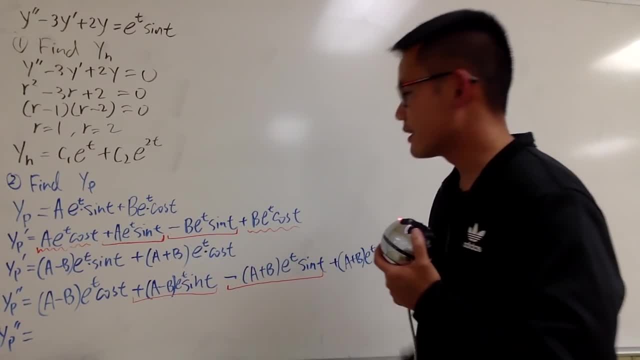 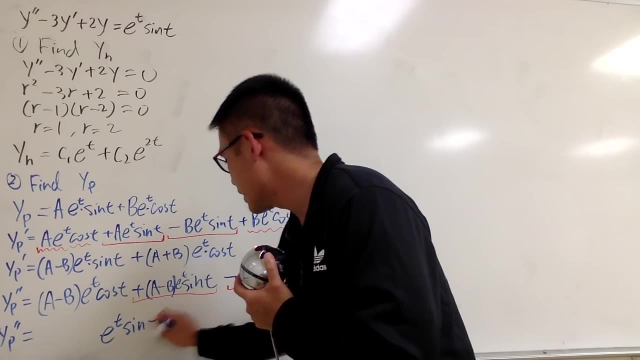 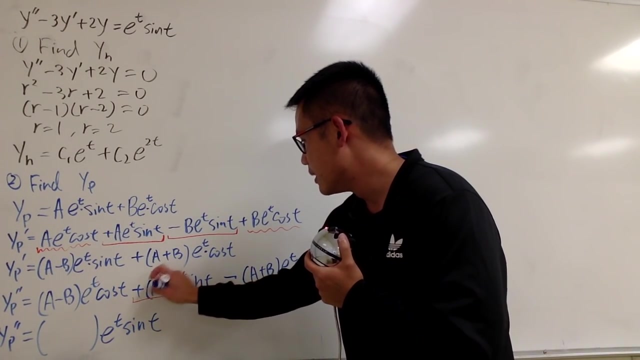 in the middle like this and that right. So allow me to just put down right here e to the t sine t first, and then I will figure out the coefficient right in the front. Okay, so do it carefully. This is positive a times. 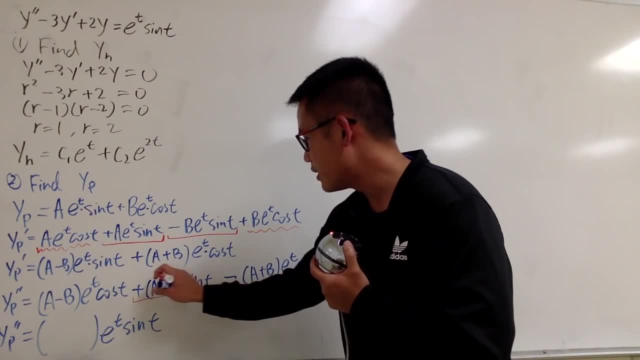 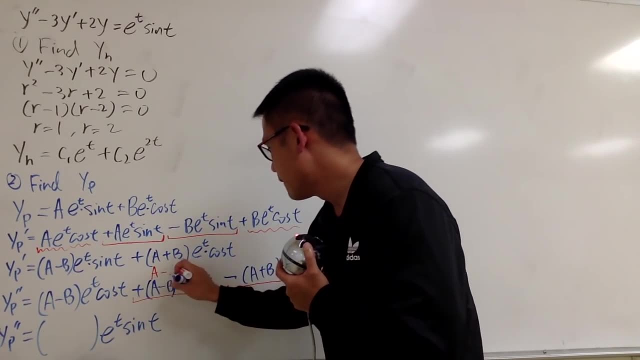 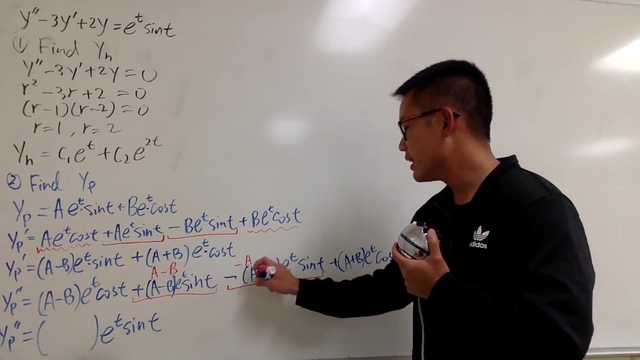 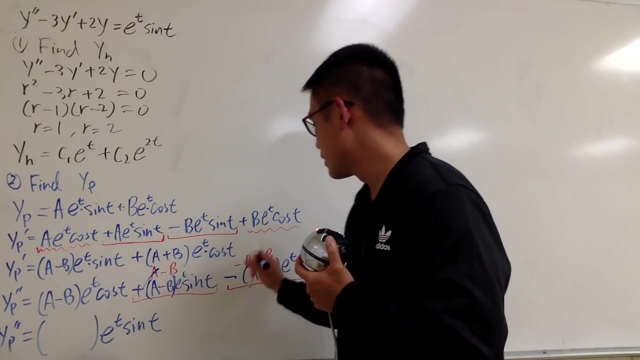 positive times, negative b, right. So this right here is going to be a minus b. okay, This is a minus b, like that. But when you distribute the negative in here, this is going to give you negative a And then negative b, right? So, in other words, you see this a and that a will cancel, and 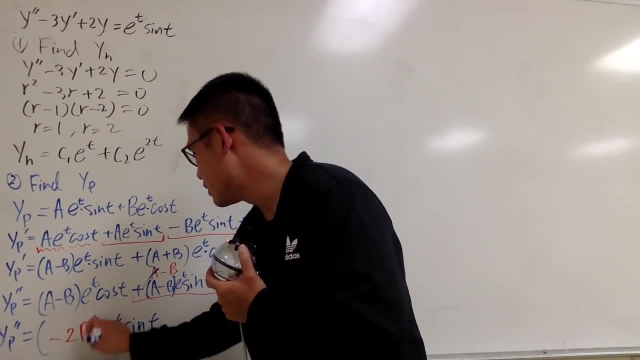 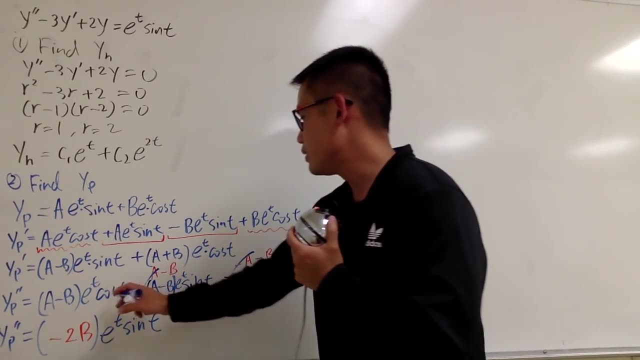 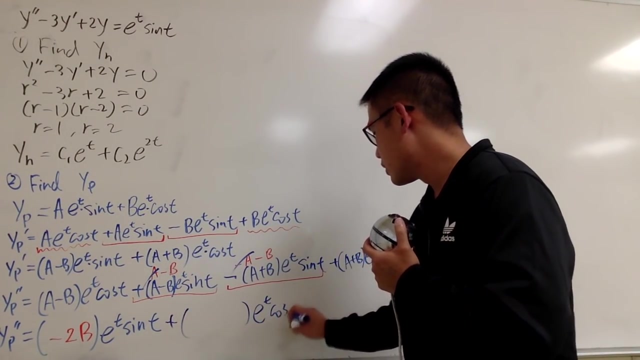 then negative b, negative b will be negative 2b, and that's the coefficient in front of this term, the second derivative, And we do the same thing for e to the t cosine t. so let me just open the parentheses for the coefficients in a minute and we will have e to the t cosine. 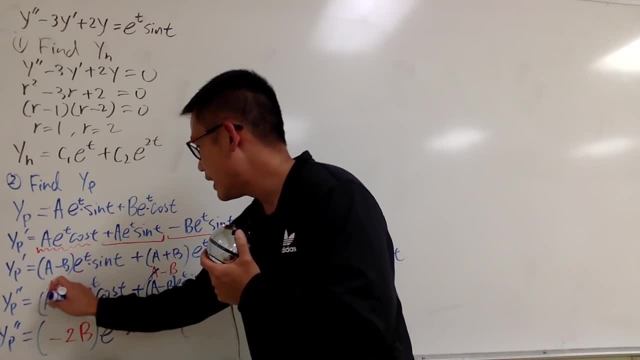 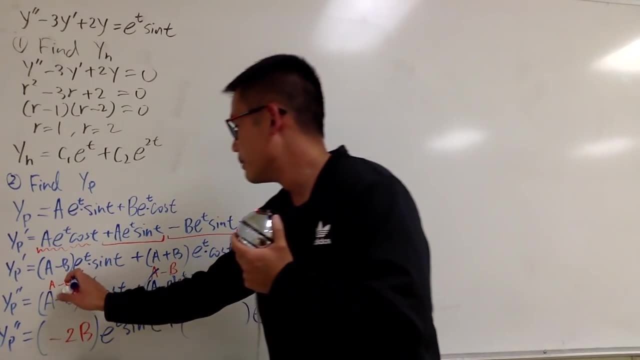 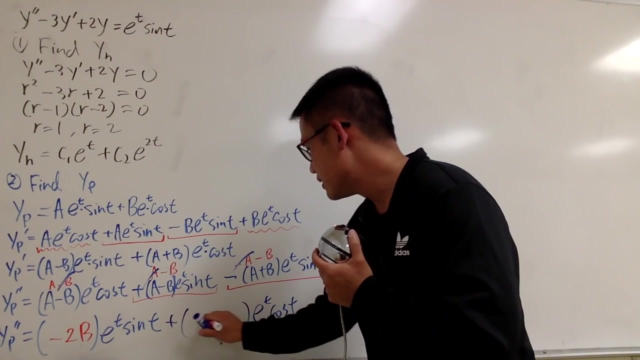 t like that. Here this is just a minus b, nothing special. and right here this is also a plus b, nothing special. but you see, minus b plus b, cancel and we just have a plus a, which right here. 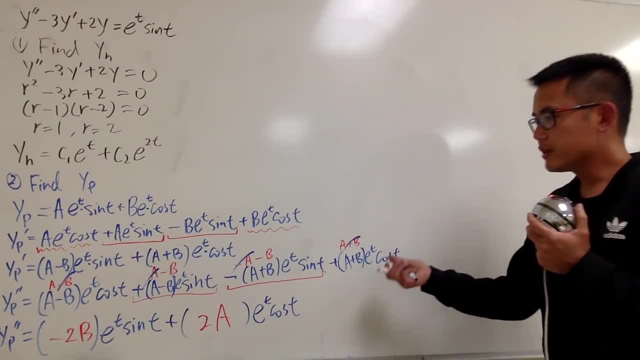 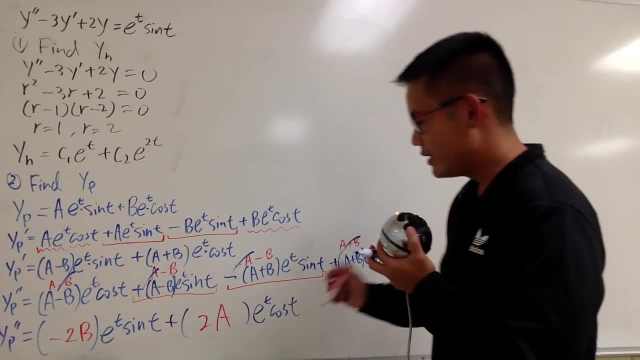 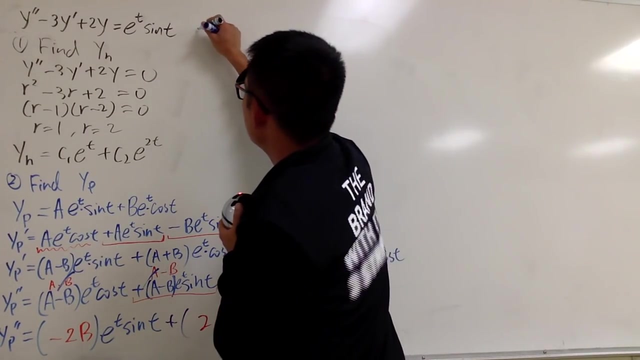 this is 2a. okay, So, in fact, the second derivative is actually better than the first derivative, isn't it? Anyways, here we go. We will plug in everything into the original. Okay, All right. So now I'm just going to draw an arrow like this: 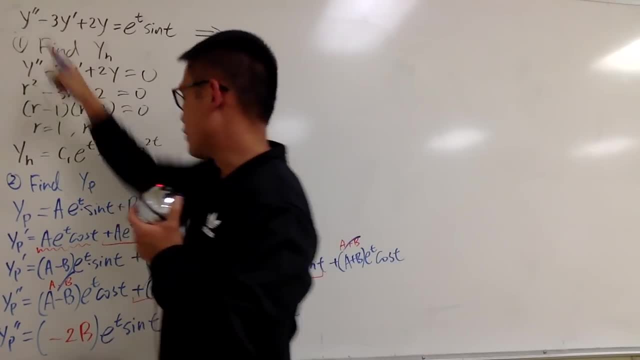 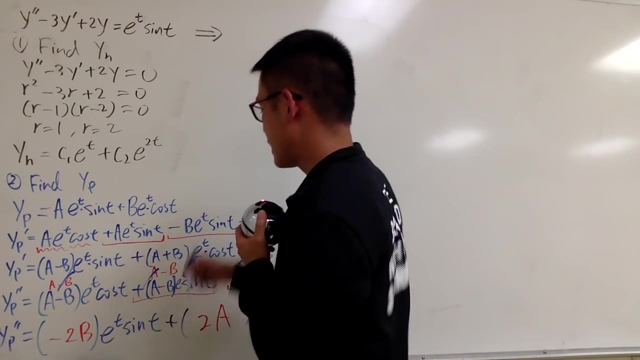 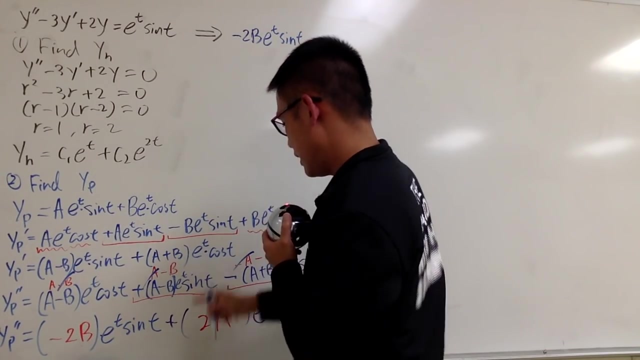 So plug in yp For the second derivative. I will just do that right. I will put this down in blue. So this is going to be negative 2b times that. so let me just write it down: Negative 2b e to the t sine t. and then we add it with 2a e to the t cosine t. 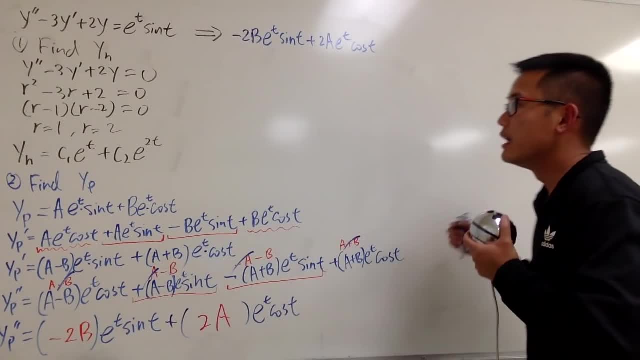 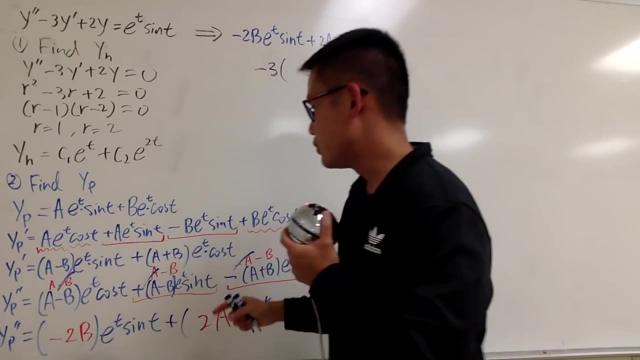 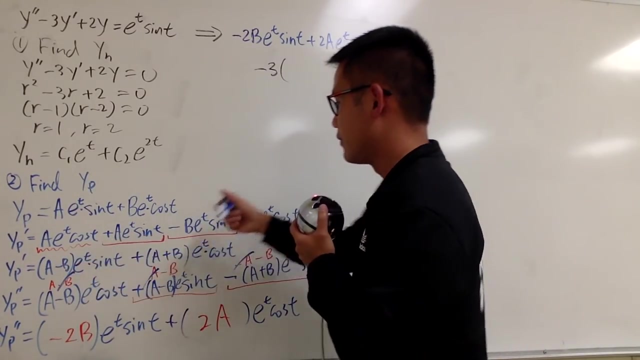 This right here is for the second derivative right, And we will let me just write down the next line: So minus 3 times the first derivative, which is this right here? okay, It's this right here and I will just have to write it down for you guys, right here. 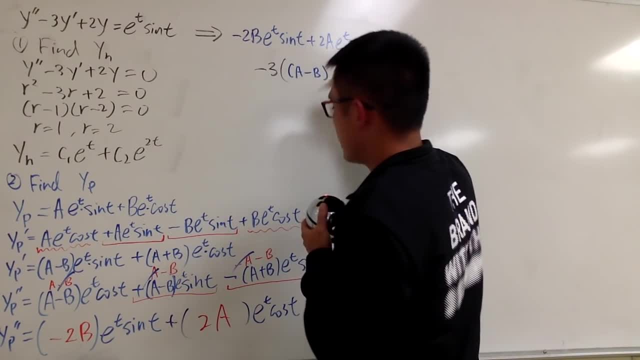 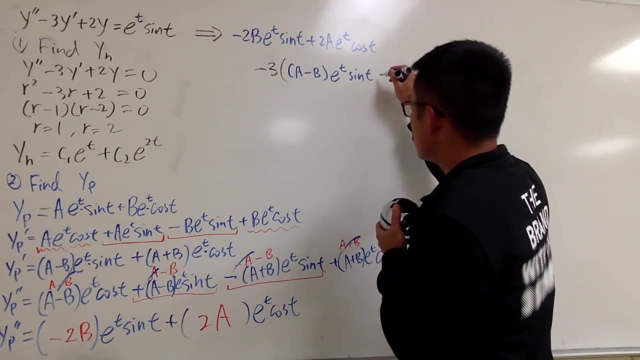 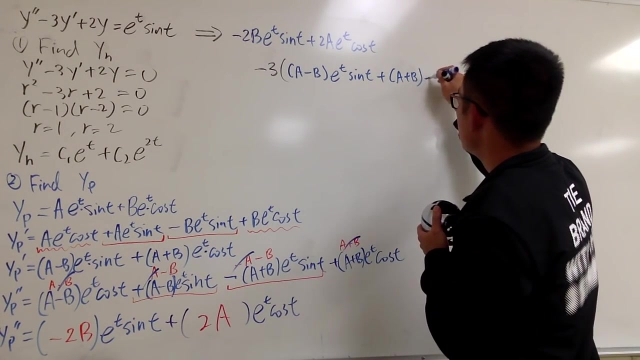 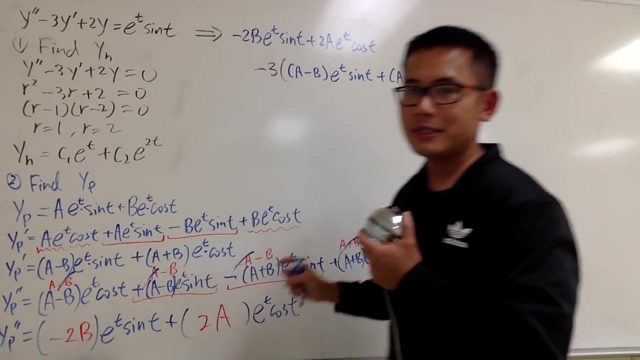 This is going to be a minus b, and we have the e to the t sine t, and then we have the plus a plus b and we have the e to the t cosine t, like this, like that, right. And then this is for the second term, like that. 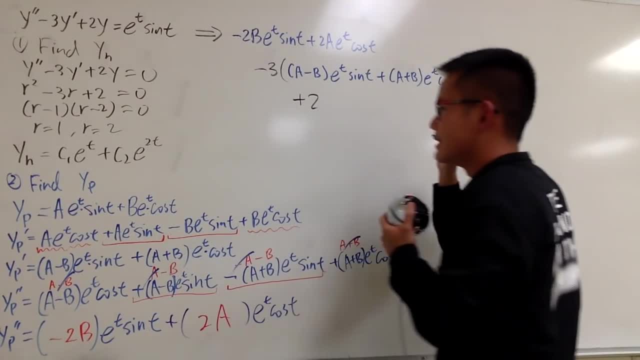 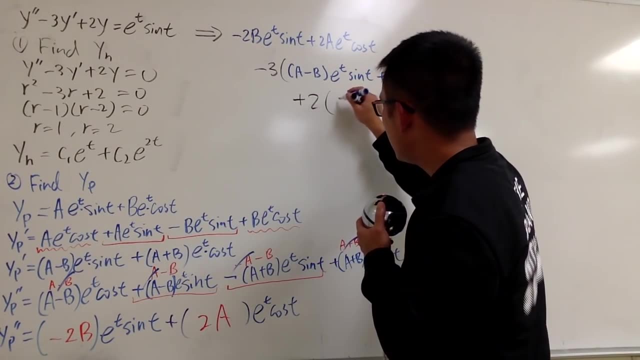 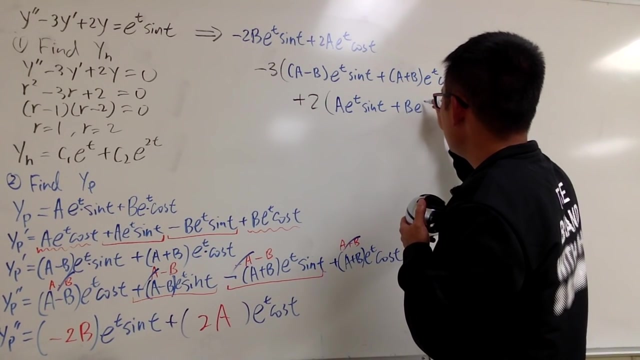 And we have to add 2 times y, which is we have to plug in yp. so it's 2 times that, which is a, e to the t sine t plus b. Okay, All of this shall be equal to e to the t sine t. 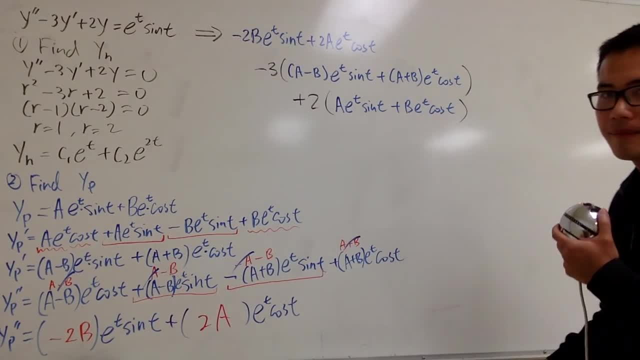 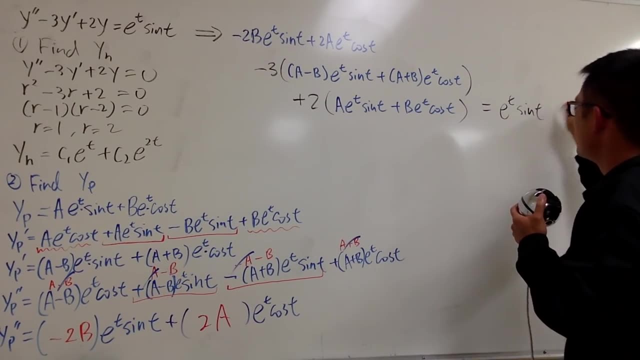 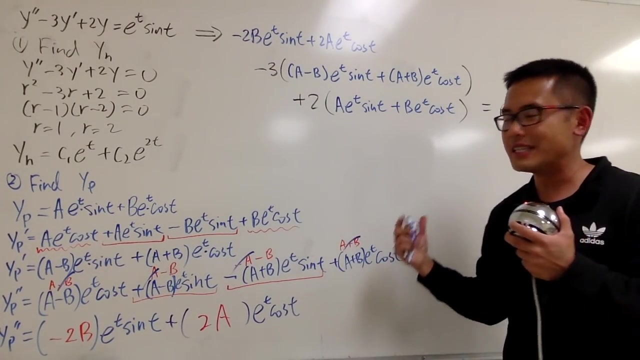 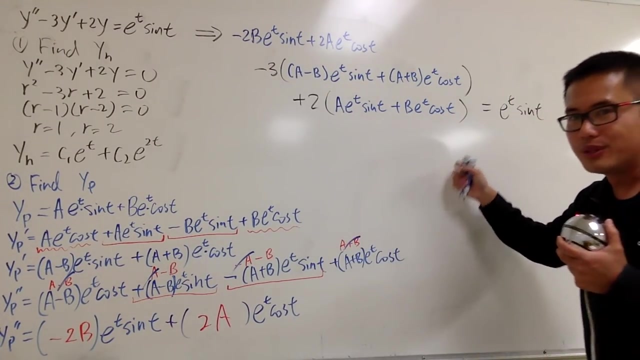 Okay, now, on the left-hand side, you know, you can collect enough terms so that you have something times e to the t sine t and likewise something e to the t cosine t, and that's what we have to do right here. 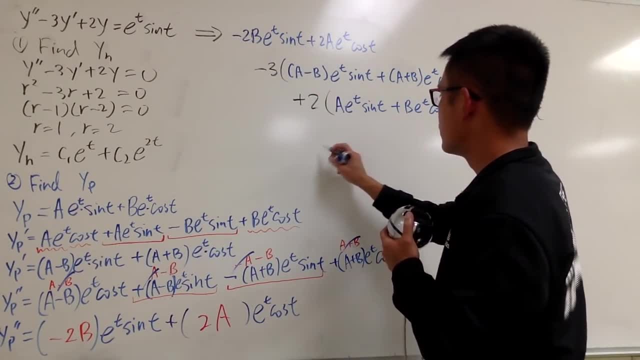 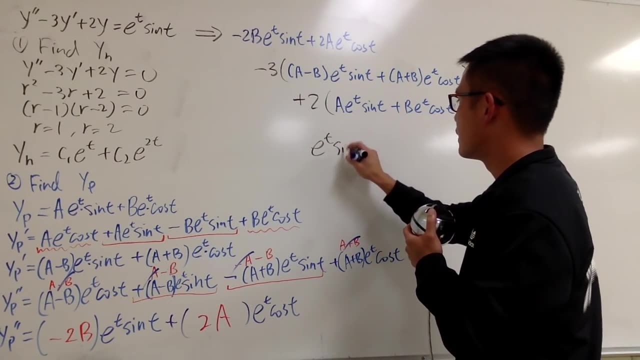 So this right here is what we have to do, and let me just set it up first. Let's look for all the terms that have e to the t. Let's put down sine t first, right, I'm not sure what's in the front yet, and then we'll add it with something, and we have 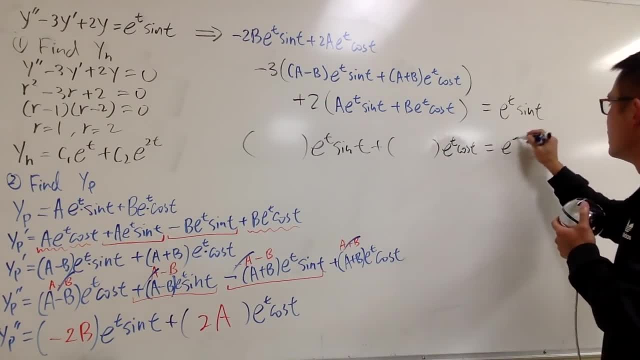 e to the t cosine t and this should give us this e to the t sine t. okay, And then we'll figure out what should go into the parentheses in red. so let's look for all the terms that have e to the t sine t. 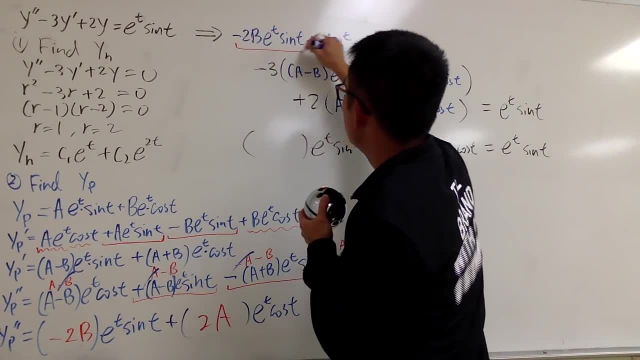 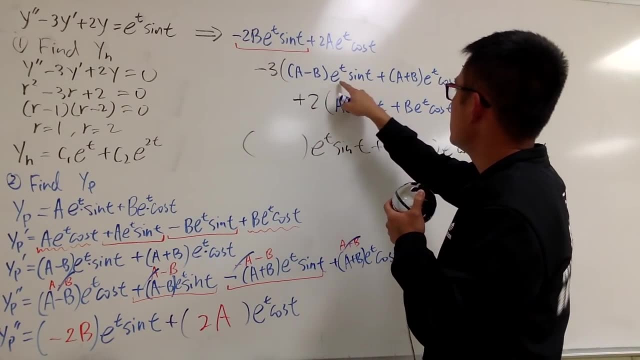 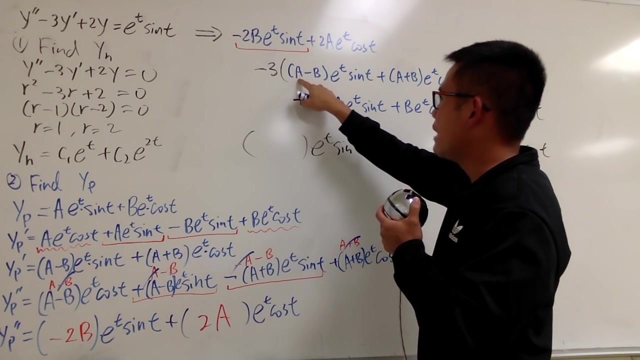 First of all, I'm looking at this right. This right here has e to the t sine t and this right here also has e to the t sine t. but then, be sure, you see, we have a times negative, sorry, a minus b, like this, but we have the. 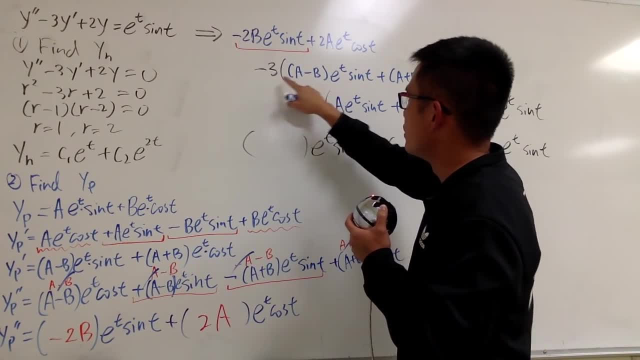 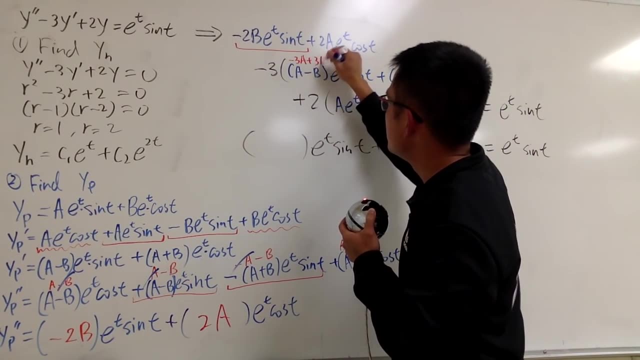 negative 3 in front. So be sure you take negative 3, distribute negative 3 times a. this is negative 3a. negative 3 times negative b is plus 3a. Okay, So I'm looking at this term now. 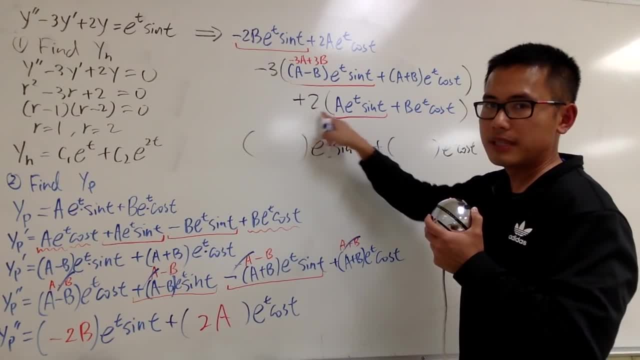 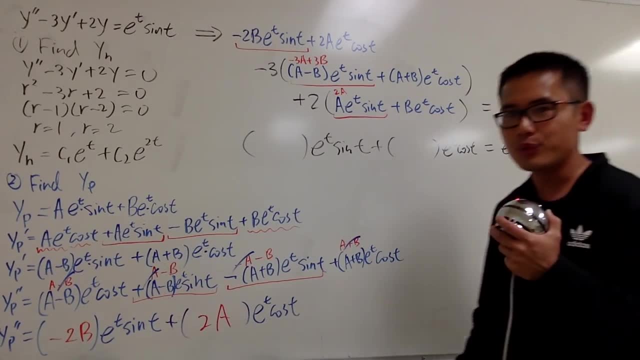 And lastly, we have this right here as well, and we have to multiply this by 2.. So I'm just looking at the coefficients. so that's just 2a, All right, so now let's see. what do we get? 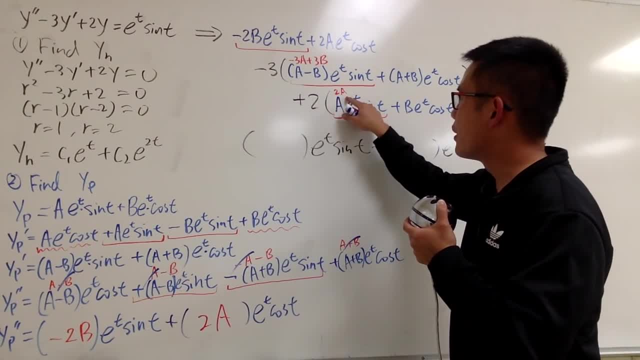 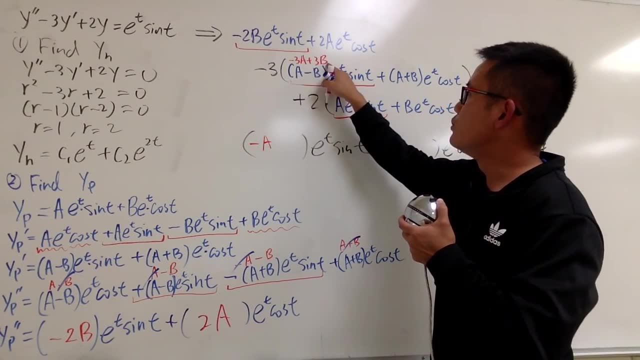 Let's collect the. a first a 2a right here minus 3a, so that's going to be negative. a right 2a minus 3a is negative a, And then 3b minus 2b. 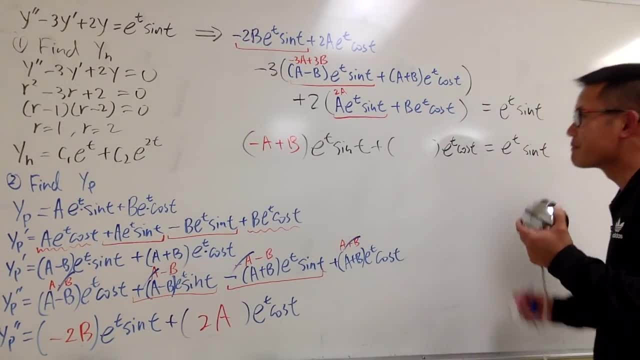 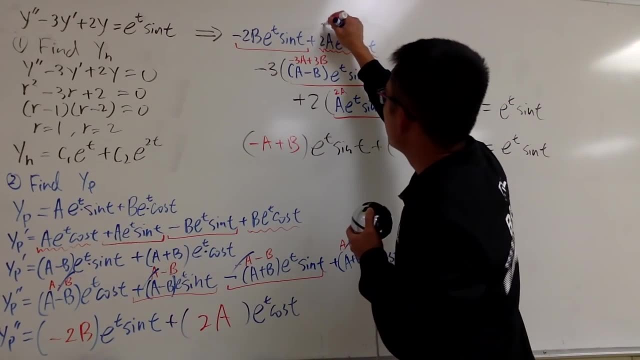 This is going to be plus 3a, So that's what we have, okay, And now we'll be looking for the et cosine t term, which is this: First I have the 2a right here. let me just make it stand out a little bit more. 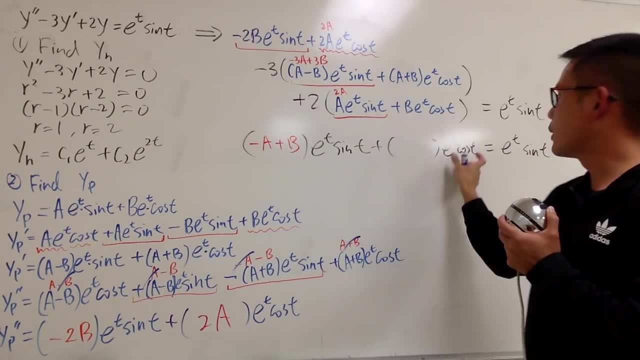 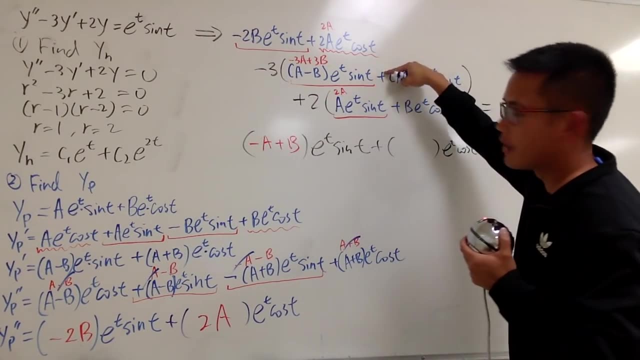 And then next, you have to be careful. This is the term that we're looking at. We have a plus b, but we still have this negative 3 in the front. Take this negative 3, put it here and then distribute. 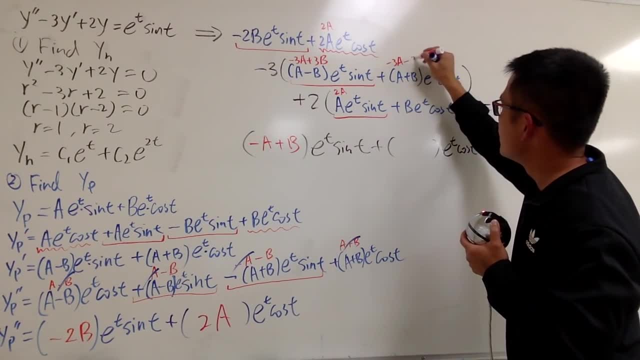 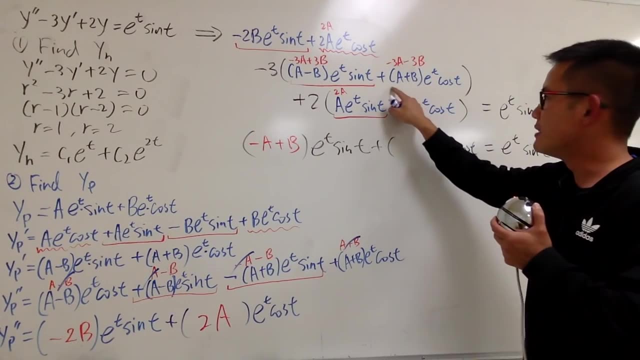 So you are talking about negative 3a and then distribute it, you get negative 3b. Like this: Once again, you have this negative 3, put it here because you have to multiply it, and then this is another parentheses. so you have to distribute right here and you get. 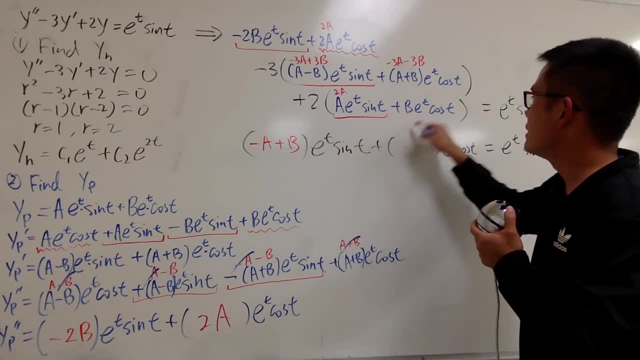 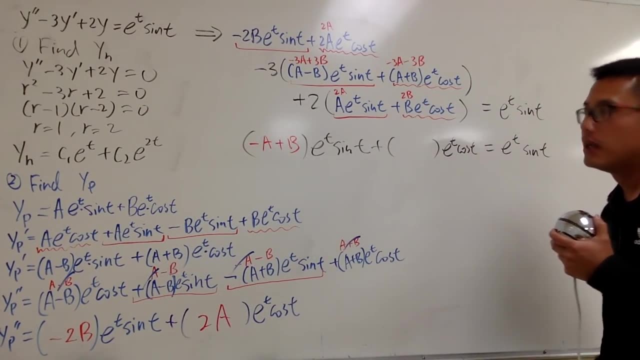 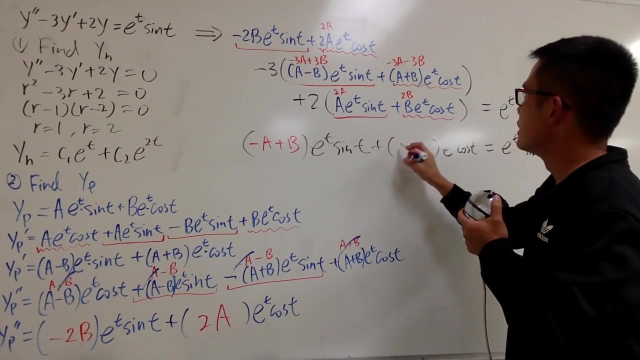 that. okay, At the end you have 2 times this, which is 2b, like that. So we're looking at this terms now. Okay, let's do the a first. We have 2a minus 3a, which is negative a again. 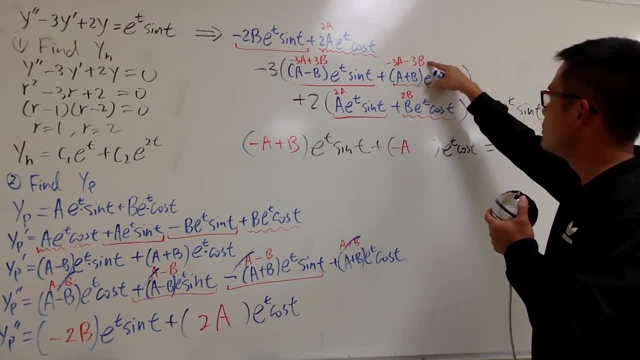 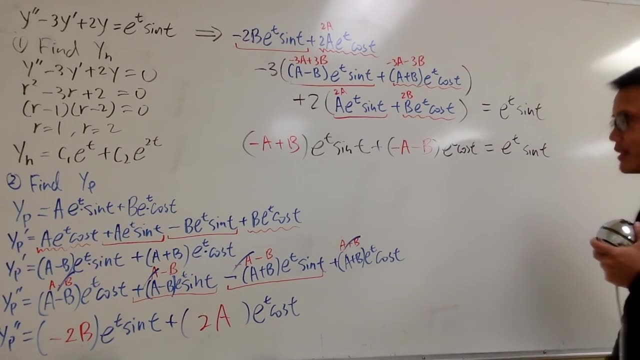 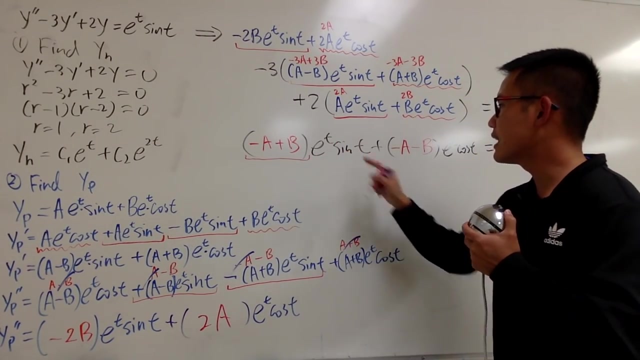 And then this and that together, negative 3b plus 2b is negative b, like that, isn't it? So this is very exciting, because now you see this right here, this is the coefficient for e to the t sine t. 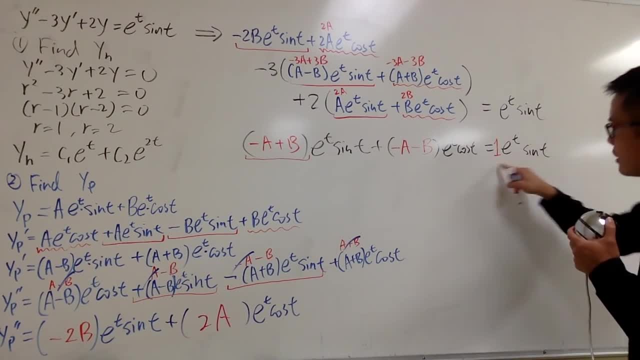 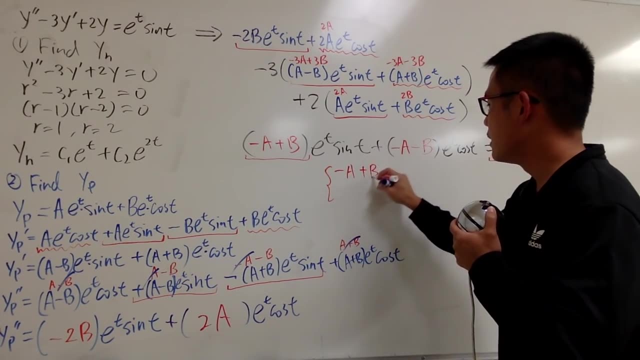 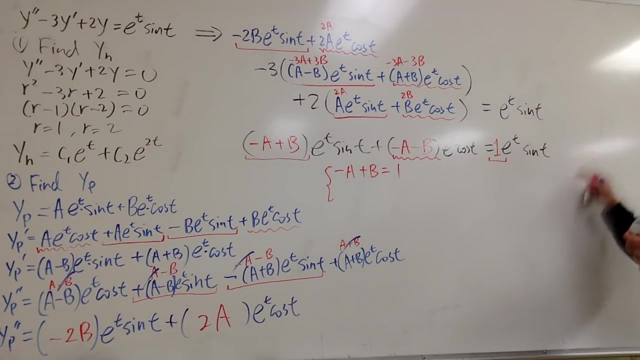 That must match with 1, because the coefficient right here is 1,. okay, So what you're saying is that you must have negative a plus b equals to 1.. Okay, And this is the coefficient for e to the t cosine t, but we don't have any right here. 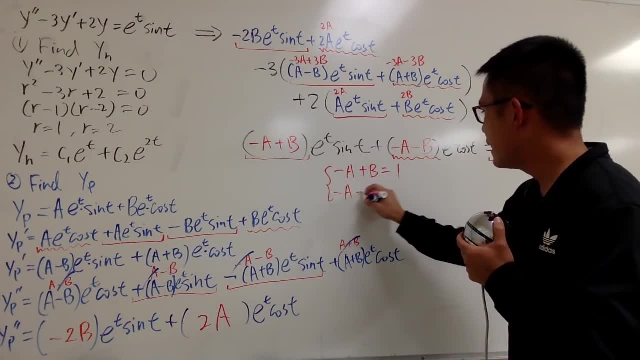 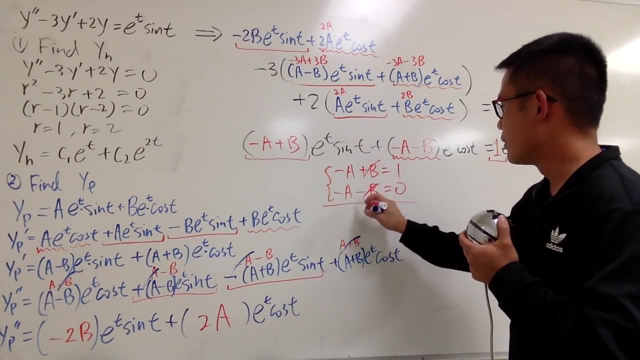 That means it's 0.. So I'll put down: negative a minus b equals to 0,. all right, And you can just go ahead and do this real quick. You see, you can just, you know, combine them. you get negative 2a, that's equal to 1, right. 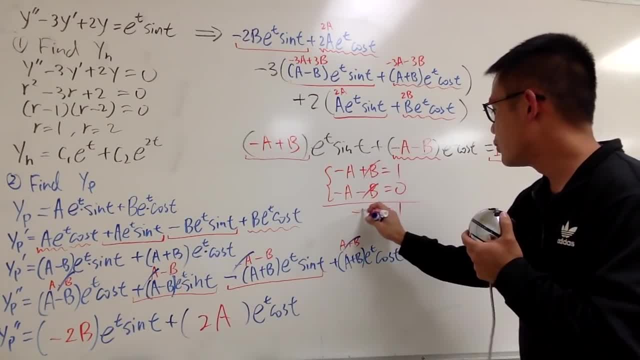 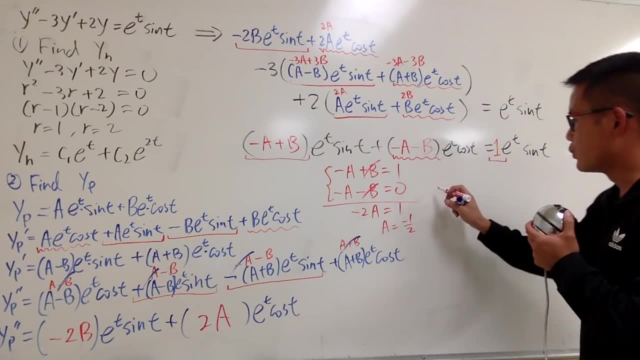 And let me just write down my 2 better. This is the negative. 2a is equal to 1.. So, in other words, a is equal to negative 1 half. Plug in negative 1 half into maybe this one. So we are talking about negative 1 half. for the a minus b- I don't know yet- is equal. 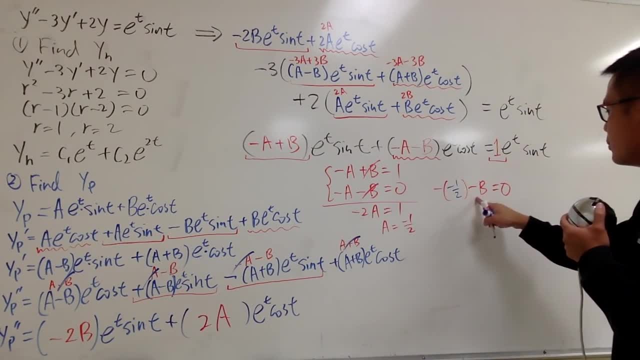 to 0.. I'm going to move the b to the other side. so you see this is going to be b, right here. Negative negative becomes positive. so you're talking about: b is equal to positive 1 half. Oh my goodness. oh my goodness. we are done with this right. 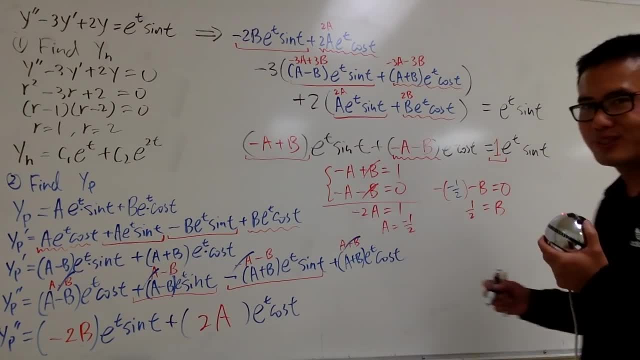 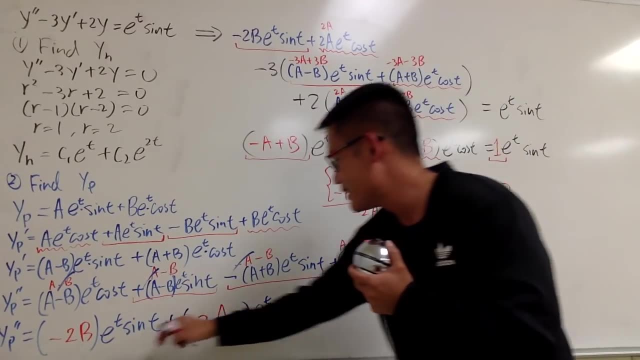 And you see, I didn't even use a calculator, So you guys can do this too. Anyways, this is going to tell you yp, or? I should still put this down in blue for the yp, right? Okay, I will. 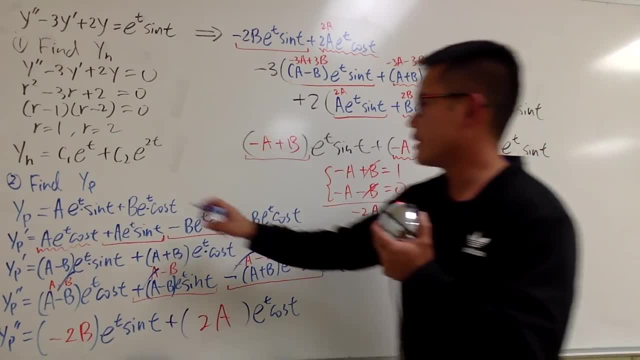 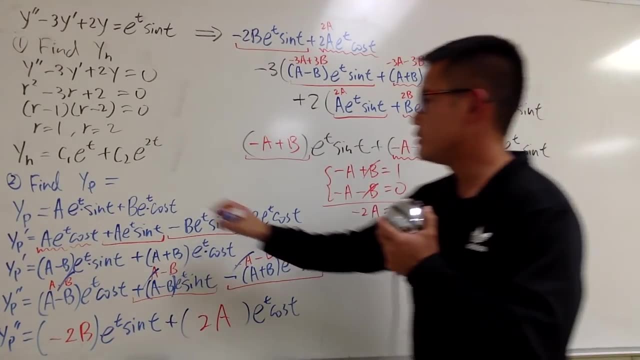 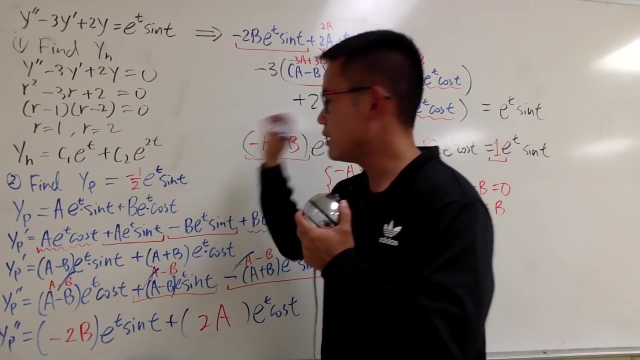 Let me just put it down here: yp- okay. Yp is going to be a. we found it which is negative 1 half, So let me just put it down right here. And then this is with e to the t, sine t, okay.